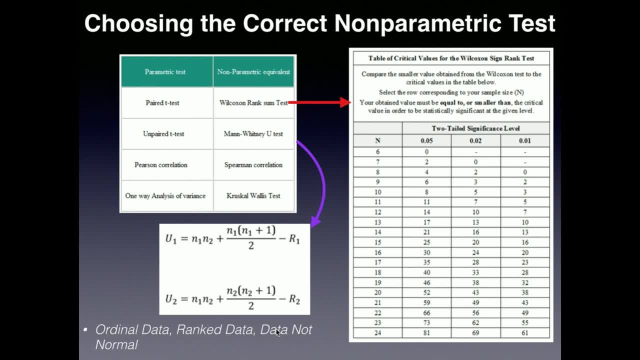 data And then, like I said, if the data is not normal, then your best bet is to use a non-parametric test. Now you can see out of the parametric ones that we've talked about a paired t-test, which is the dependent t-test. Unpaired t-test is an independent t-test. 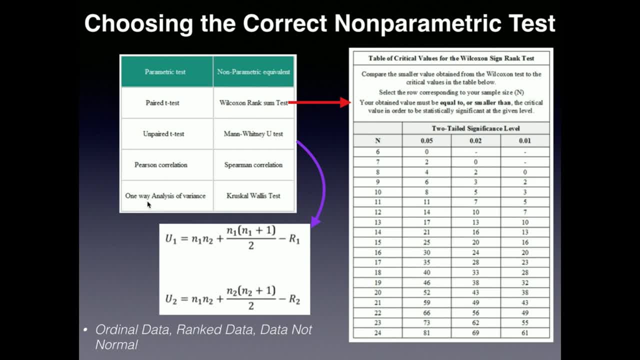 Pearson correlation. that's just normal regression that we talked about- And then ANOVAs. Each one of these parametric tests has a non-parametric test. So if you have a non-parametric test, a non-parametric equivalent. Now, if you were to look at your data and your experimental 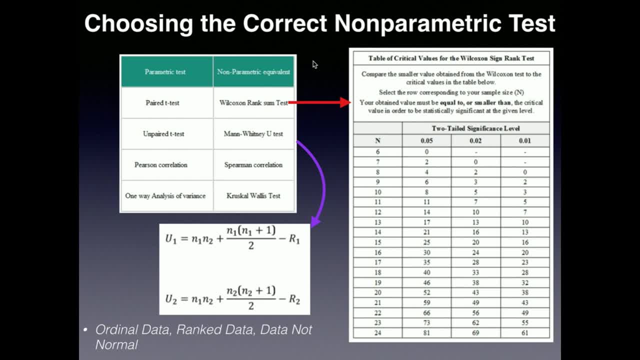 design and you determined that the appropriate statistical test could be a paired or dependent t-test. but you knew the data was not normal. then you can say: well, let's use the non-parametric equivalent of that test, which turns out to be a Wilcoxon rank sum test, And this video: 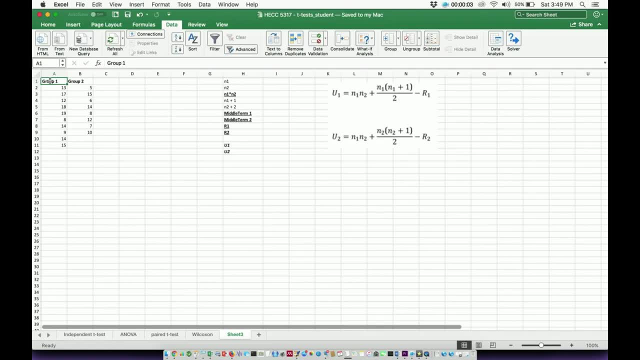 I'm going to show you how to perform a Wilcoxon rank sum test. All right, So we've got our data here and we're ready to perform the Mann-Whitney. I also have from the PowerPoint these two formulas here, which are almost identical. 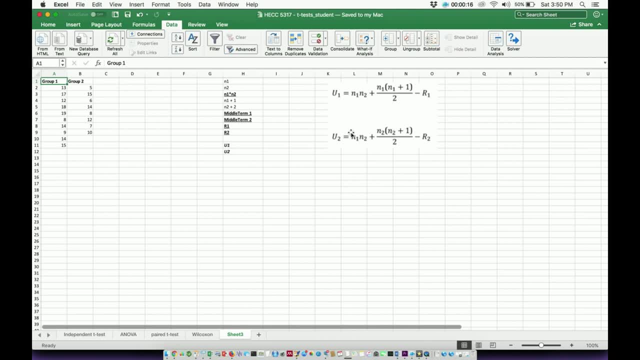 but one's for the first group, one's for the second group specifically, thus the subscripts one and two. Got my data here. two groups Again. remember this particular non-parametric test is the equivalent to the independent t-test. So remember the number of data points in each. 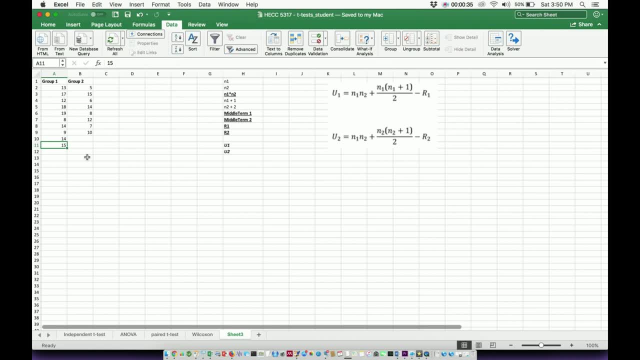 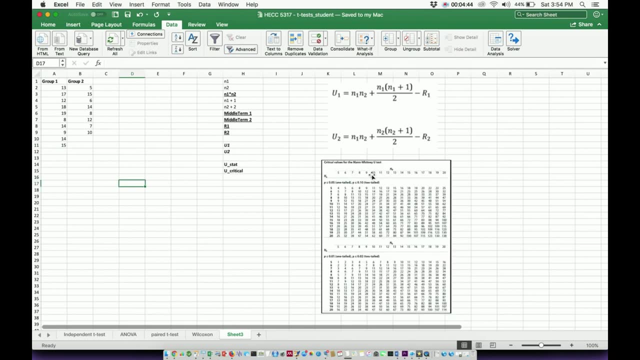 group does not have to be the same, unlike the paired t-test or its non-parametric equivalent, The Wilcoxon rank sum test, which we covered in the previous video. I've also just added this table of critical values that we're actually going to use first to determine some of these. 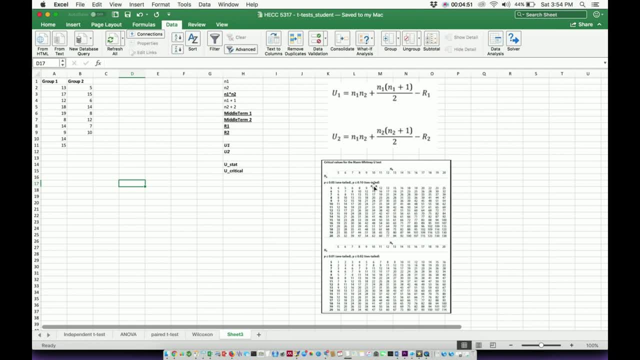 important things over here before we do anything else. Now they use the terminology here n sub a and n sub b. We're using the corresponding n1 and n2, but it's the same kind of thing, All right. So first of all, n1, this is actually the number of samples that we have in group one. 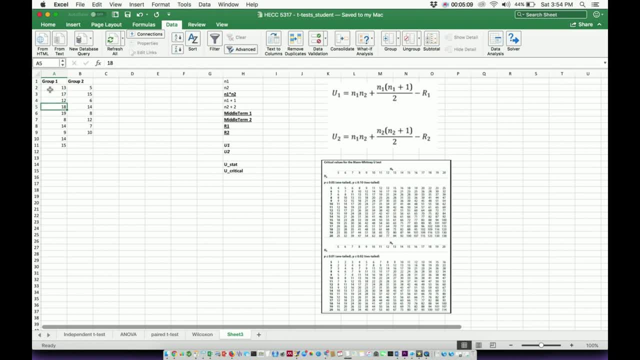 So let's actually determine this: One, two, three, four, five, six, seven, eight, nine, 10.. So our n1 here is going to be 10.. For n2, it looks like eight, but let's just verify this: One, two, three, four, five, six, seven, eight, All right. 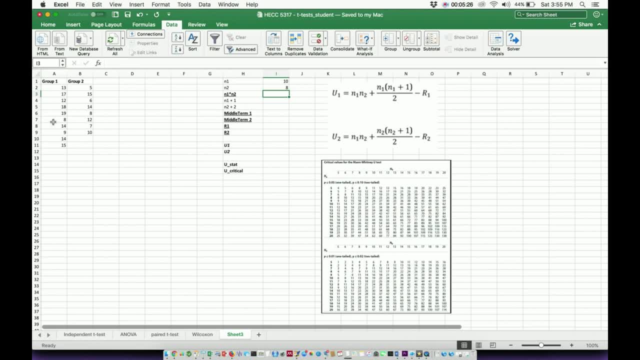 Very quickly. if you have a very large data set, there's actually a way that you can do this actually very quickly to count these up. One of the things you can actually do is if you have the data analysis tool pack installed. if you don't, I have a video. 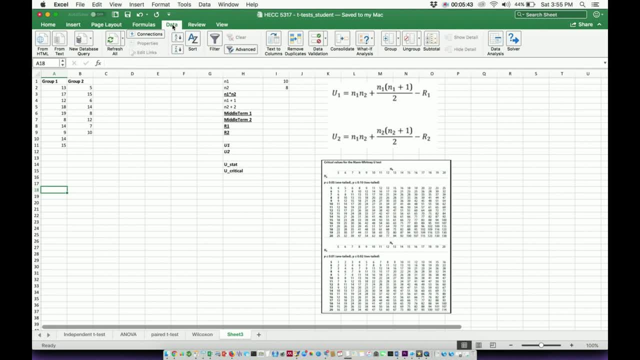 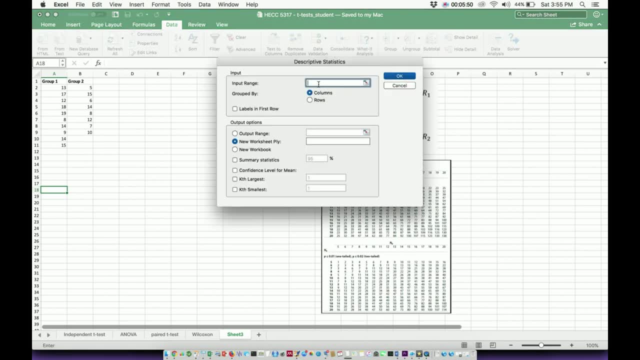 that I'll put in the description here to link to it where I discuss how to install it. But you would go to data data analysis and you can actually go to descriptive statistics And I can go ahead and, just for one of these columns, input this in and put my output right. 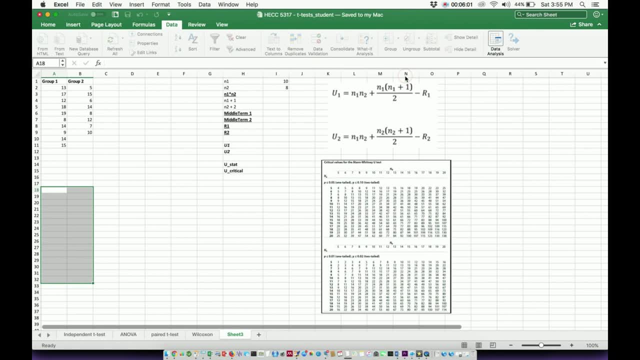 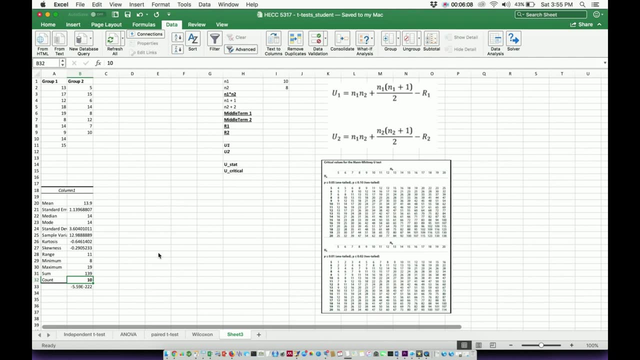 here, Let's do summary statistics. We don't really need that, but you can see that the count tells you right, there is 10.. Okay, Now, I don't need that here, Although I'll just leave it, but that's a way that you can actually add these up. 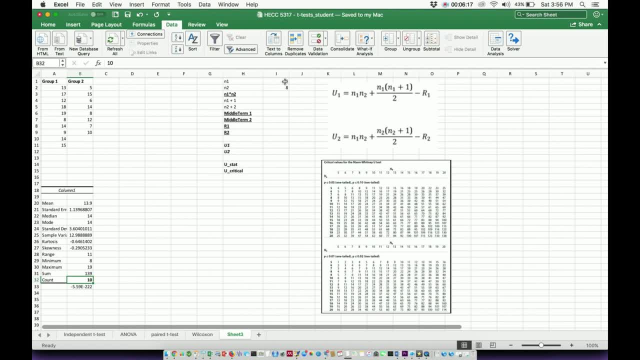 see how many you have very quickly. All right, So I have this now. Now I need to do n1 times n2.. Now the reason I'm doing this and I bolded it is because that's one of the important terms in each. 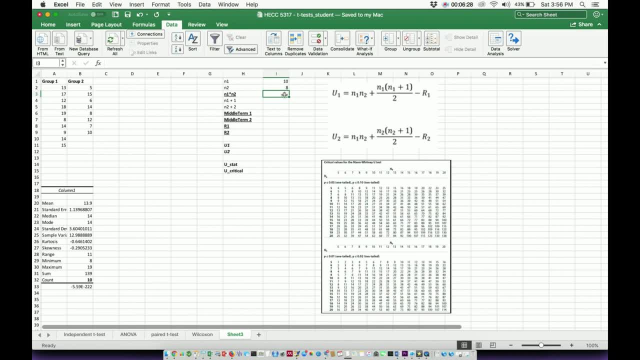 of these U calculations. I need to multiply these two together. Now I think we can all do 10 times eight in our head, but I'm going to go ahead and program this, just in case it was a very large or weird numbers. So I'm going to go ahead and program this, just in case it was a very large or weird. 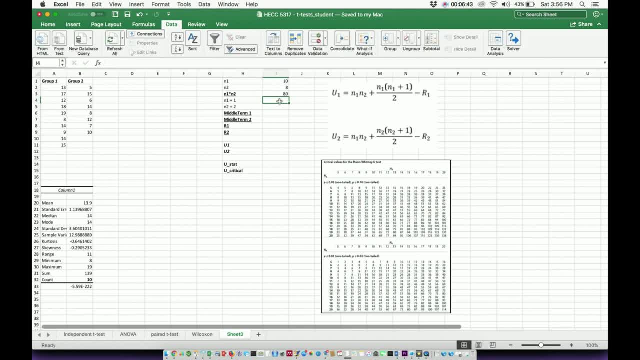 numbers. So I'm going to go ahead and program this. just in case it was a very large or weird numbers, So I'm going to get 80 there. Okay, Then I need to do these two things: calculate n1 plus one. 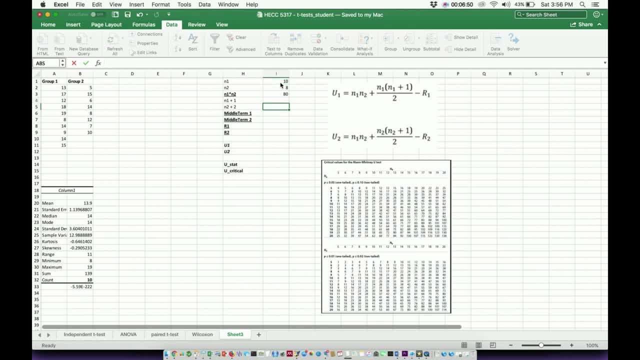 So I'm going to take n1 plus one. All right, That's pretty self-explanatory. I just like programming this. So n2 plus one- this should actually be a plus one right here. So that's eight plus one is nine, And what I can now do is calculate this middle term right here. 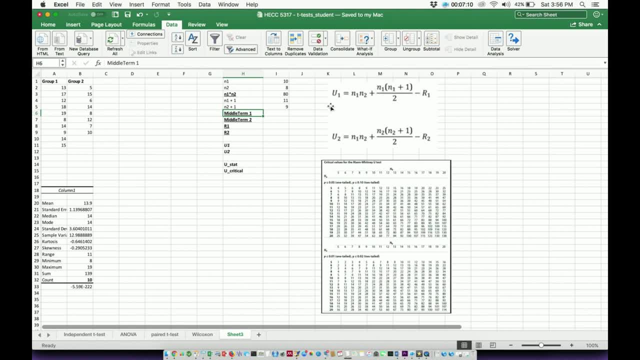 This is going to be the quantity n1 plus one. So I'm going to take n1 plus one, which is this one right here, times n1, and then I'm going to divide it by two. So I'm going to do equals and what I'm going to do is, in parentheses, this n1 plus one, okay, times n1,. 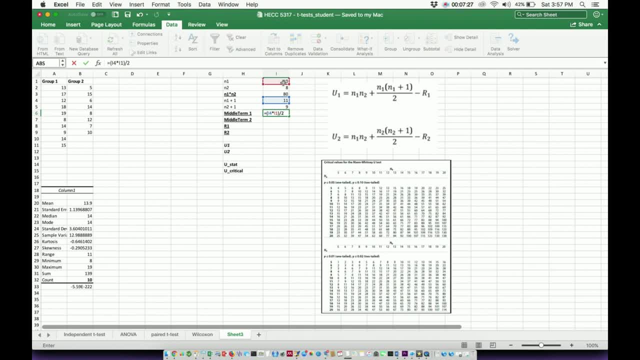 close parentheses and then I'm going to divide that whole thing by two as it tells me. All right, That gives me 55. That's my middle term for the first one. Now I need to do the same thing with the n2s. So again, hit an equal sign here. open up our parentheses, do this n2 plus one, and then I'm going to divide it by two. 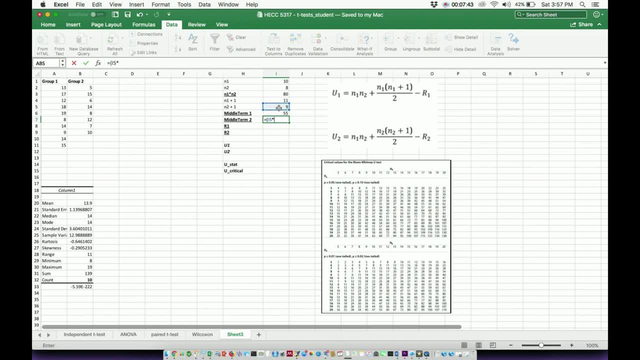 So I'm going to do n2 plus one and then I'm going to multiply that times n2, my eight, then divide the whole thing by two, as it tells me, and I get 36 here. for the second middle term, We now need to calculate r1 and r2.. And to do those we're going to use this data right here now. 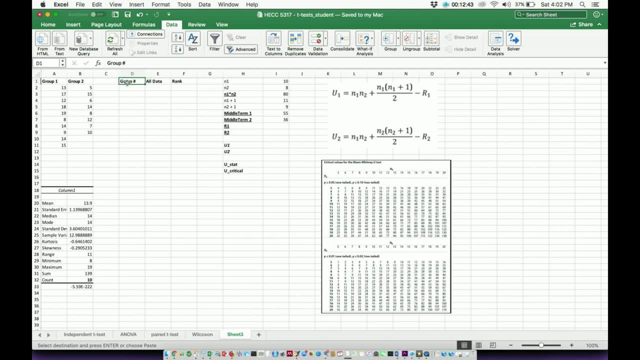 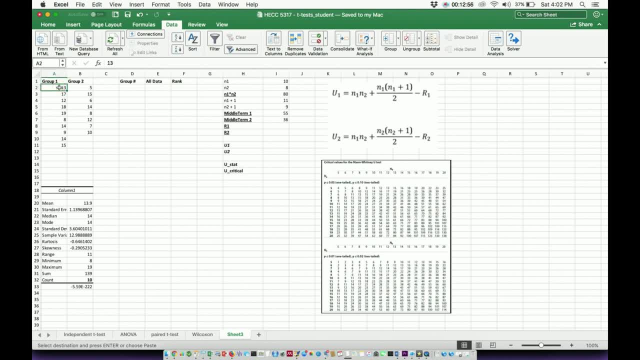 And this says rank. So what I'm going to do is I'm going to take all the data from group one and I'm going to put it under all data. All right, Then, because these belong to group one, I'm just going to put a one in front of all of these. 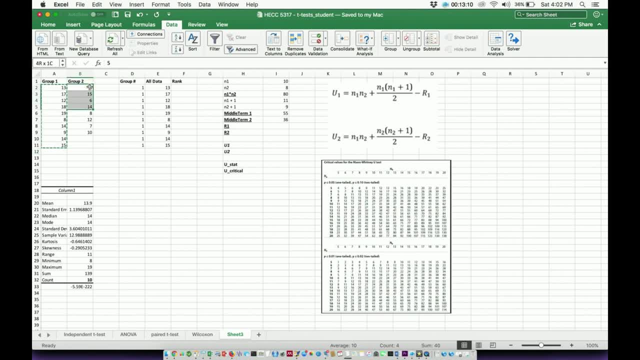 Okay, Now I'm going to do the same thing for group two. Take all of this data, copy it and now paste it under this one column, And these belong to group two. so I'm going to put a two in this column for all of these, Oops, Okay. 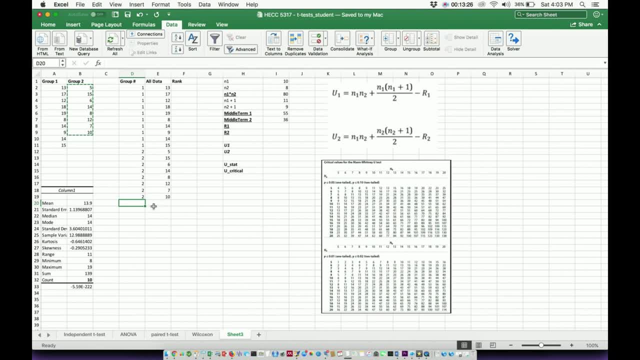 So now I have all the data in one group, which is what I want to do, because in a Mann-Whitney U-test, even though these are two groups of data, when you obtained them to do the analysis, you have to assume they're all from one group, so you have to put them in one column. 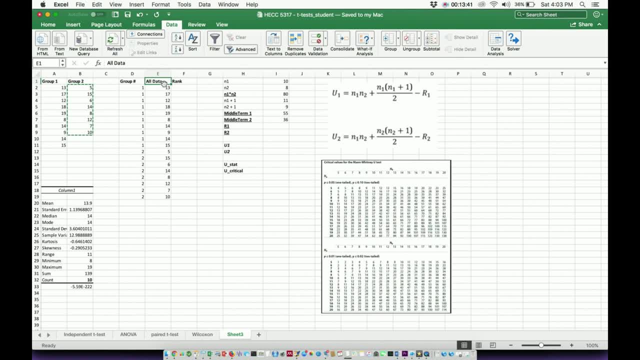 So now what I'm going to do is I'm going to put my mouse on all data, I'm going to highlight this cell and, assuming I'm under the Data tab, I'm going to click Filter. Now you'll see that I now have these arrows for group all data and rank. 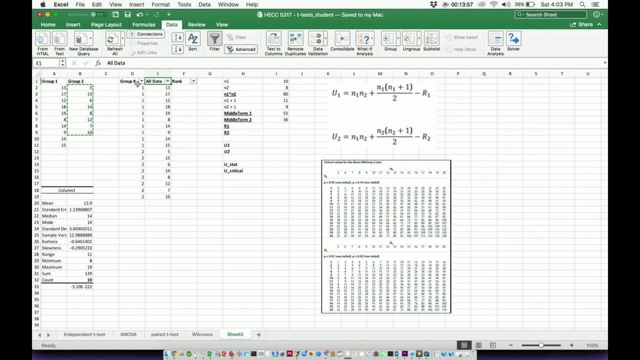 It's very important that you have it for all three of these, especially the group number and rank. So now you see, I have these arrows for group number, all data and rank. It's important that you have it for all of these, all three of these. 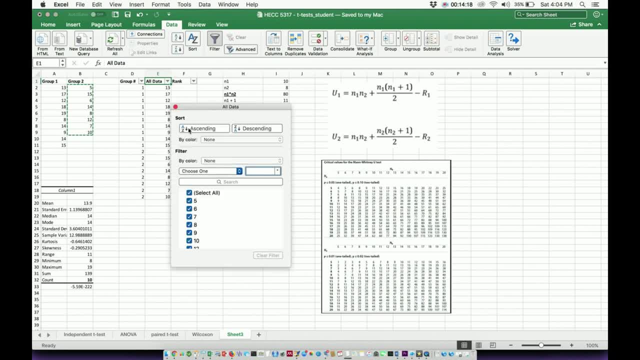 So what I'm going to do is go to All Data, click on this arrow and I'm going to sort these in ascending order. So I click on Ascending and you see what happened. It orders them from the lowest. It orders them from the lowest to the highest number. 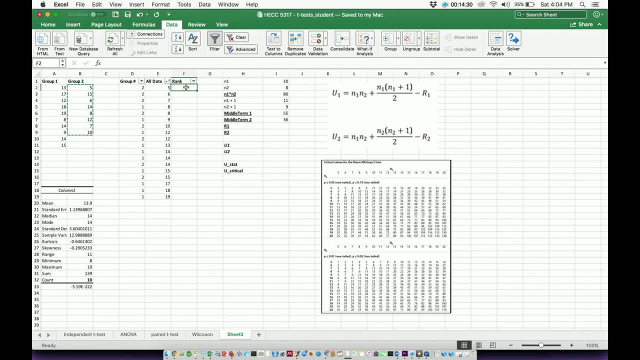 So what I'm going to do is, now that these are in order, I'm going to rank them, starting with one at the lowest, and then just go in order. There is probably a better way to order these with Excel, with some function. 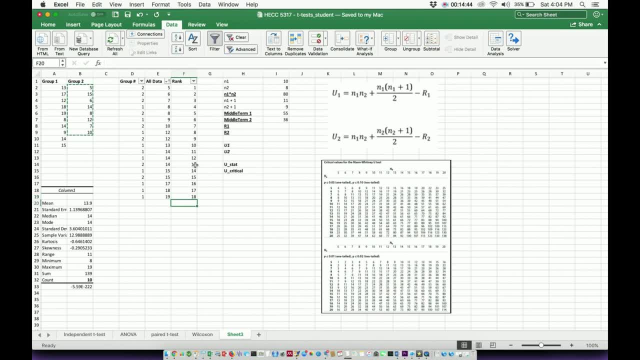 I'm honestly not sure what it is, But the point is you rank them like this: Now these are ranked. What I need to do to calculate R1 is add up all of the ranks. The problem is they are now all out of order. 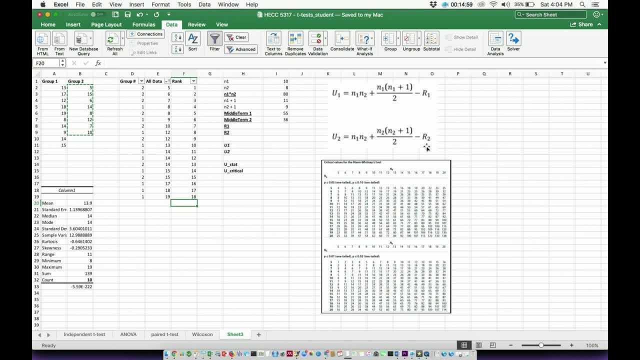 I'll do the same thing for R2.. I need to add up all the ranks for group 2.. Here's why I had you put the 1 and 2 in front of here, Because now we can go back to this arrow and sort them in ascending order. 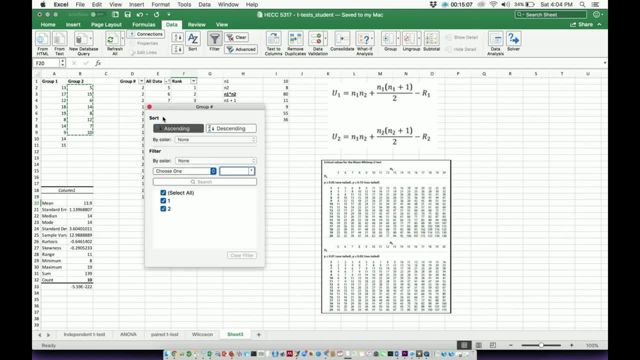 And now all the ones are together, And it also kept the ranks with them. All right, So to calculate R1, let's do equals program function sum. I'm going to do the same thing for R1.. I'm going to do the same thing for R2.. 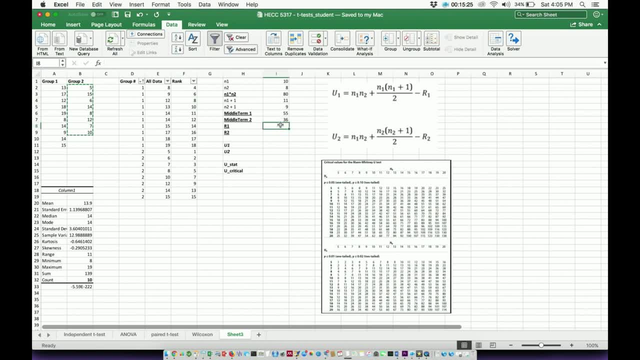 I'm going to do the same thing for R1.. I'm going to do the same thing for R1. I'm going to do the same thing for R2.. I'm going to do the same thing for R1.. I'm going to add up all the ones associated with group 1.. 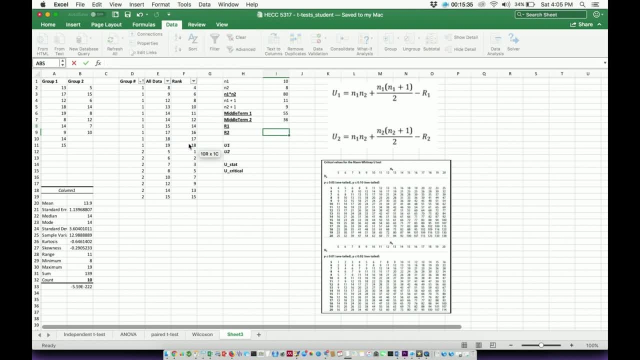 That's these right. That's these right. Hit enter. So there's my R1.. My R2 equals: Let's program another one. Let's program another one. I'm now going to add up all the ones that are associated with group 2.. 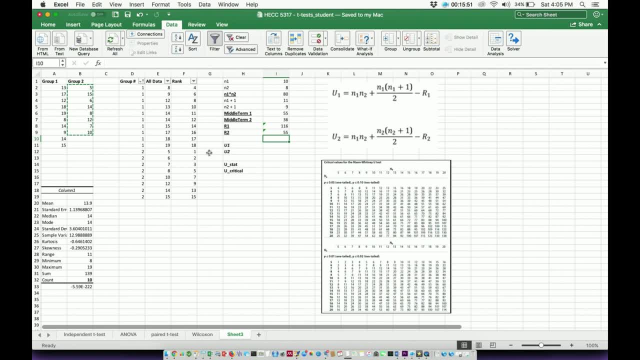 That's my group- 2s Enter And that R2 ends up being 55. And that R2 ends up being 55. So now I can now apply these formulas. So now I can now apply these formulas: term and then subtract the corresponding r. So let's calculate these u's Equals. I need to take: 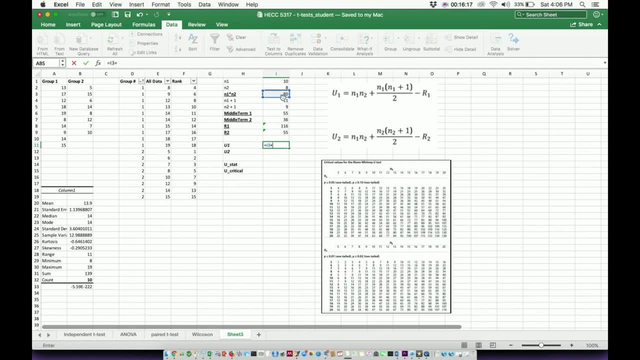 the n1 times n2,, which is the same for both of them, add the corresponding middle term- this is going to be middle term 1, and then subtract r1.. Enter. That gives me a u1 of 19.. Now I'm going to. 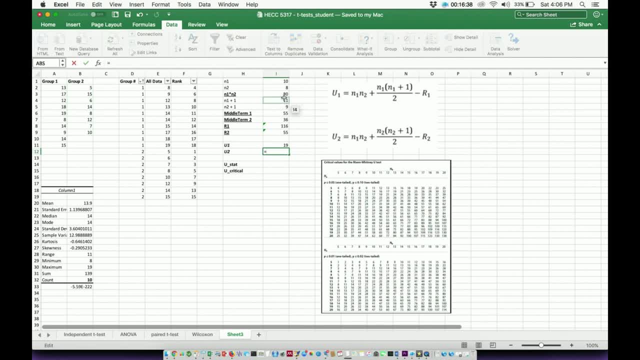 do the same thing for u2.. I'm going to take this n1 times n2, I'm going to add the middle term- this is middle term 2, and then I'm going to subtract r2.. Equals and I get 61.. The rule is: 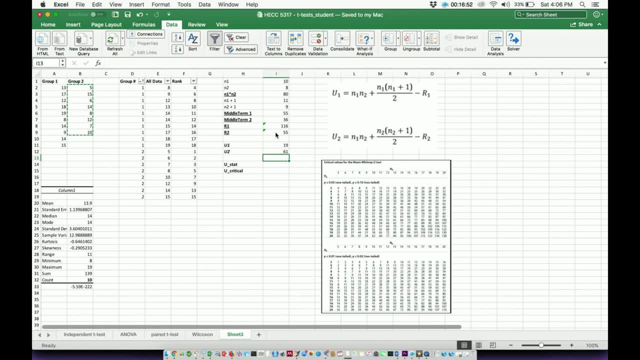 is the u that you use is always the smaller one. So my u1,, therefore, is the important one here. So that means my u statistic is 19.. I can find these Mann-Whitney u-test tables on Google. just type in the Google keywords. We're going to assume a 90% confidence level. so our p or 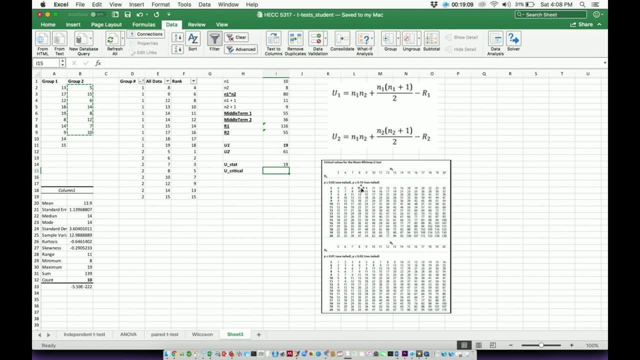 alpha value that we're. our critical value is going to be, let's see, 0.10.. So we're going to use this top table up here. Our na, that's our n1,, that's the nomenclature we're using- is 10.. So let's scroll down to 10.. Our nb, or n2, is 8, which we see right. 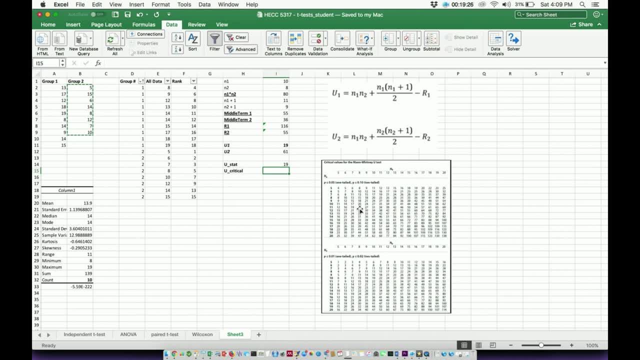 here. So what I'm going to do is scroll over to 8,, and it looks like my critical value of u is 20.. So now I have everything I need to determine whether or not these two groups over here are statistically different or not. The way I'm going to think about this. 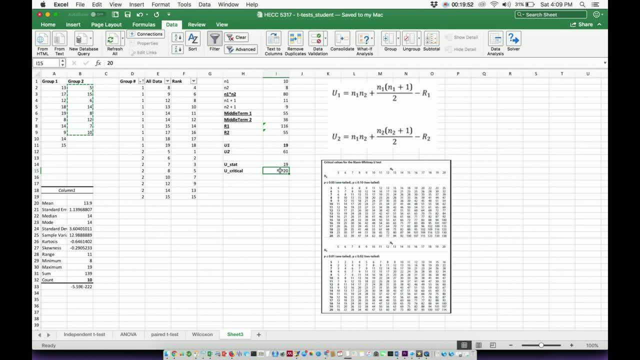 is this critical? u is like the alpha value, It's like 0.05.. This u statistic is like my p-value. Remember, if the p-value is less than .05, it was significant. If it was greater than it, it's not. So I say, is my U-statistic greater than or less than the critical u? Well, in this case, 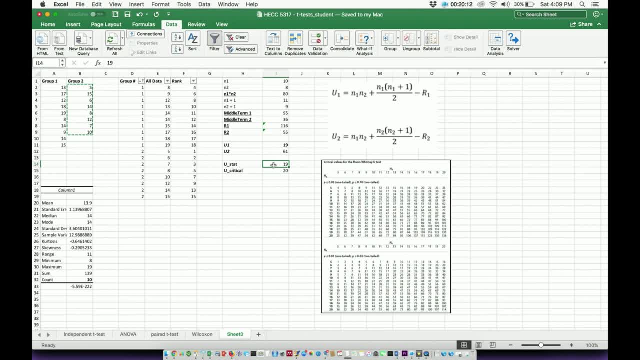 the? u statistic is actually less than the critical value. That means I reject the null hypothesis and that means my difference is is significant. I reject the null hypothesis because u-statistic is less than the critical? u. If this? u-statistic had been greater than the critical? u then I would not be able to reject the? 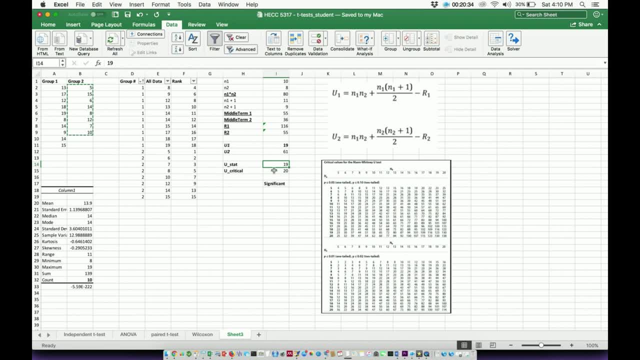 null hypothesis I would fail to reject, and then there would be no significant differences between group 1 and group 2.. Okay, so pretty much this is a more tedious test to calculate by hand than the Wilcoxon rank sum test, but once you get the hang of this, it's not that bad. The main thing to make.